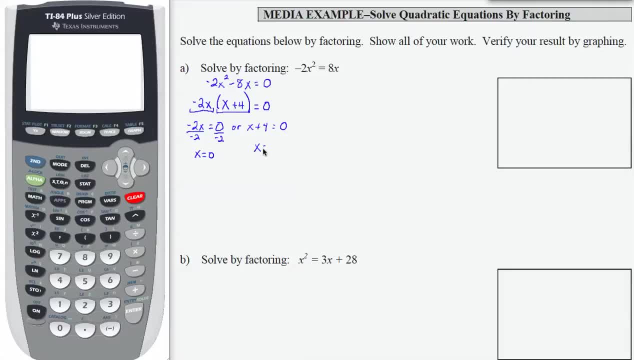 zero. if I subtract 4 from both sides, I get a result of x equals negative 4.. So I have determined two possible solutions to my quadratic equation. I'm going to use my calculator to check these solutions. I'm going to go to y equals and I'm going to clear anything I have in y1.. If my y2 is, 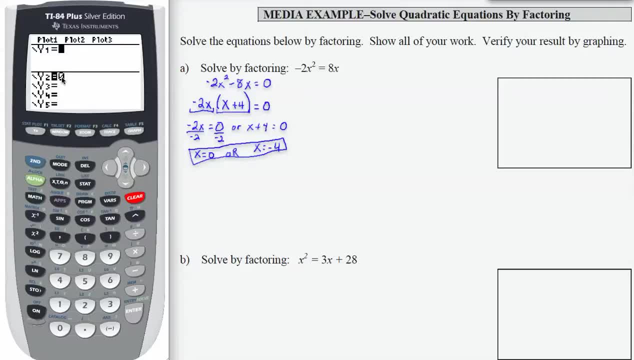 zero. I'm going to leave that. If it's not, I'm going to put zero for y2.. So what I'm going to check graphically is the solution to the equation in standard form. I could do this one, but I'm 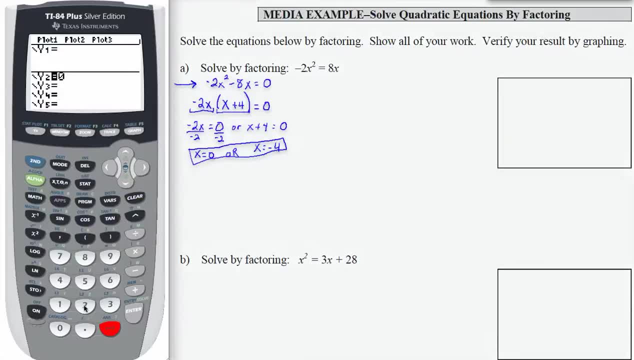 going to choose to work with the standard form equation instead. So that's negative 2x squared minus 8x. I want to check my window and make sure I have a standard window to start, then press graph Notice. I have a parabola that opens up and crosses the horizontal axis in two places. What I'm going? 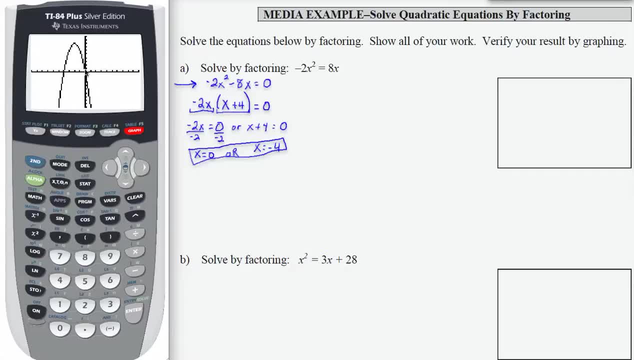 to check and make sure is that it crosses at negative 4 and 0, and that will verify my solutions. So I'm going to use my second calc intersect, which is known as the intersection, and I'm going to use my second calc intersect, which is known as the. 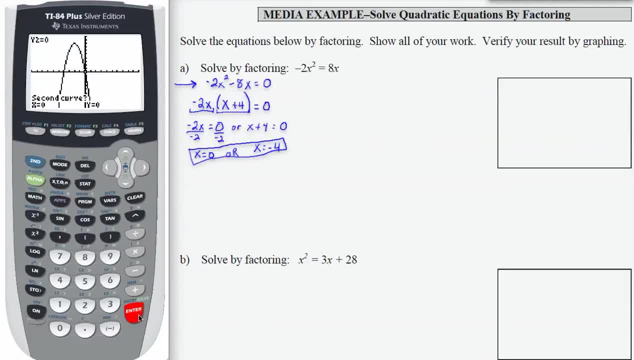 intersection and I'm going to use my second calc intersection, which is known as the intersection number 5 process. That's going to give me the first solution, the intersection 0, 0. So this x equals 0, has been confirmed. I'm going to use the same process, second calc 5, but now where it. 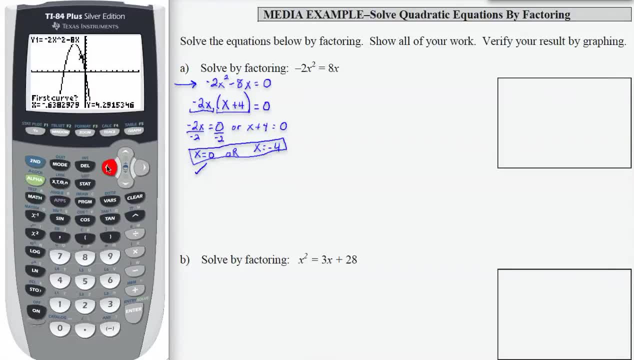 asks me: first curve, I need to move my cursor so that I can pick up that second intersection. See how the cursor is going up, Coming down. as soon as my cursor is closer to this intersection than this one, I can go through my process of hitting enter, cycling through the questions and I come up with. 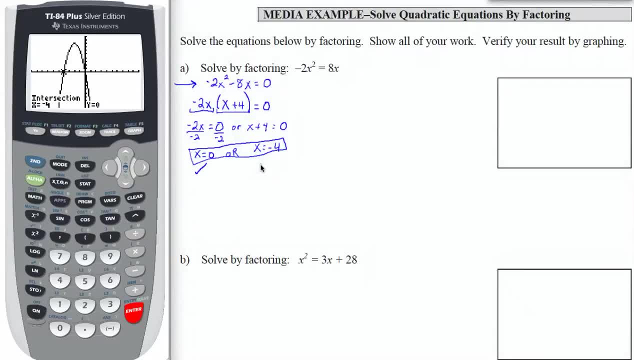 the result negative 4, 0,, which verifies this solution. So what I want to do over here in my graphing space is just to draw my axes here, my x-axis, my y-axis, and then let me get a fairly good shape on this parabola. 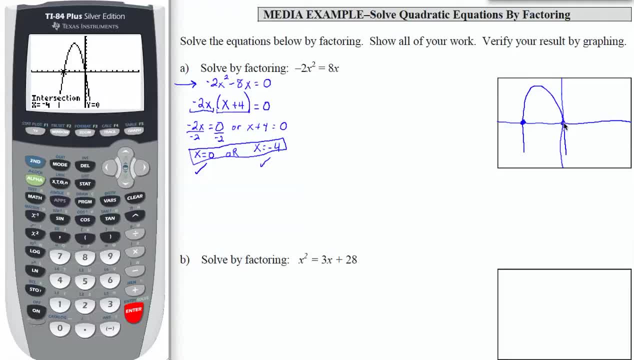 That's not great, but we can identify Those are the places my parabola crosses the horizontal intercept and that's going to be negative: 4, 0, and 0, 0.. So those crosses, the places where it crosses the x-axis or the horizontal axis, are the 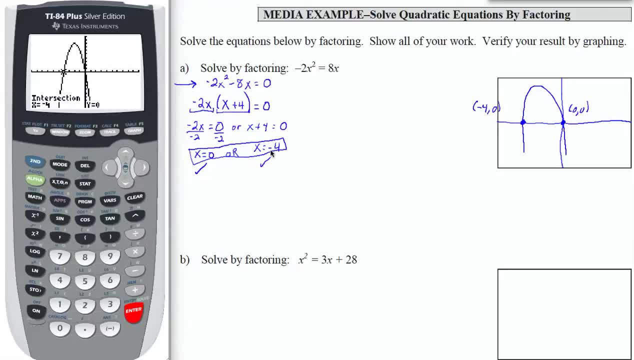 ones that verify my solutions to the equation. All right, let's look at the same kind of process for the second part. x squared equals 3x plus 28.. So the first thing I'm going to do is to set this in standard form by subtracting 3x and. 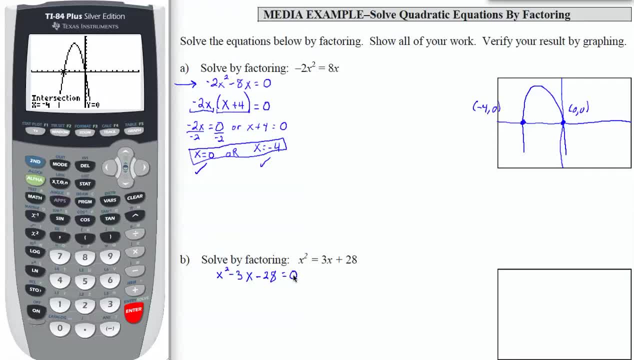 28 from both sides. So I'm moving everything to one side and putting 0 on the other side. Now what I'm going to do? I'm going to go ahead and put in my y equals equation. So this is going to be x squared minus 3x minus 28.. 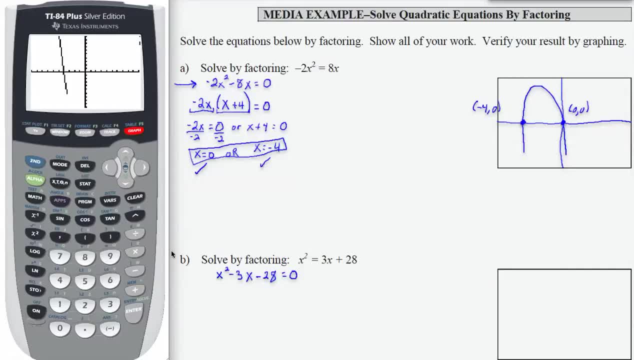 I know my window is good. I'm going to press graph and that's going to give me a parabola that opens up. I'm going to draw that here And I've got something that is Going about like this. I'm not really worried about getting the vertex in here. 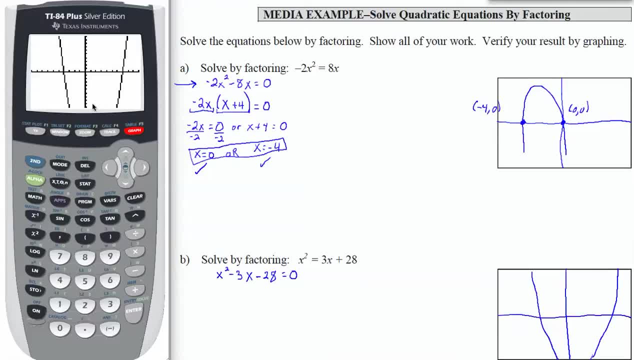 I could get the vertex if I wanted to make my window a lot more negative for y min, But I'm just going to leave it, because what I'm really concerned about is these two crosses the place. it crosses the horizontal axis here, So I'm looking. 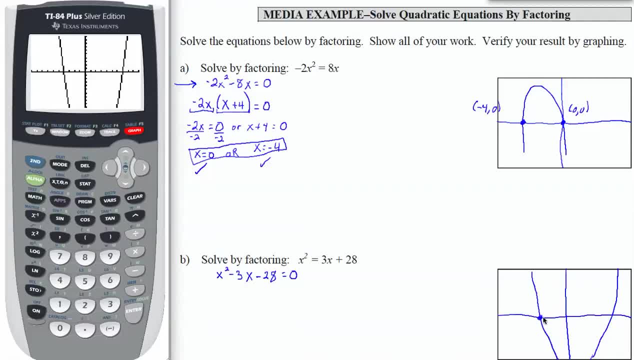 And I want to factor this to try to find these. Let's see These solutions here. Where does it cross these intercepts? So what I'm going to do is I'm going to try trial and error factoring. So I want these two numbers to multiply to give me negative 28, and add to give me negative. 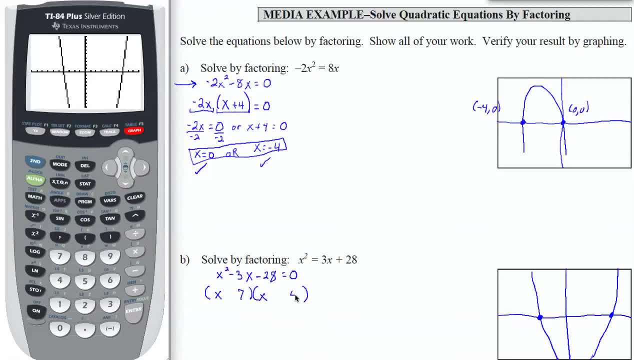 3. Well, 28 is 7 times 4.. That's a really good set of numbers to start with. I could use 14 times 2. But that's not going to help me with this negative 3.. So I'm going to do that. 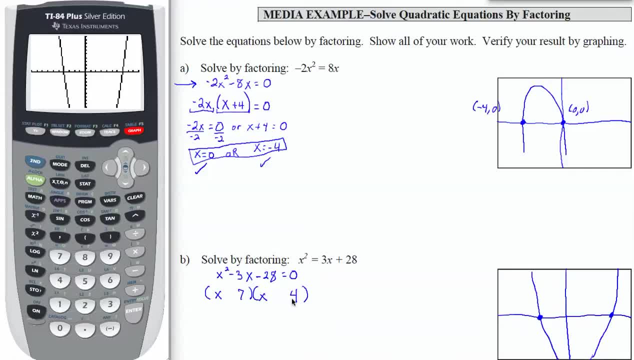 So if I want a negative 3 in the middle- that comes from adding the 7 and the 4 spots- I need it to be a negative 7 and a positive 4.. If I add negative 7 plus 4, that's going to give me a negative 3.. 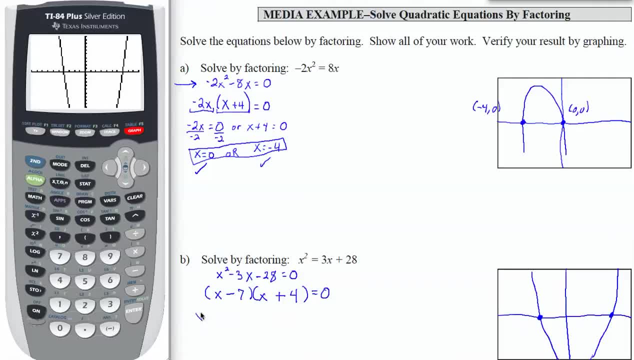 Remember to set this equal to 0.. Once I have it set equal to 0, I can set each of my factors to 0. So I have x minus 7 equals 0, or x plus 4 equals 0. That means x equals 7.. 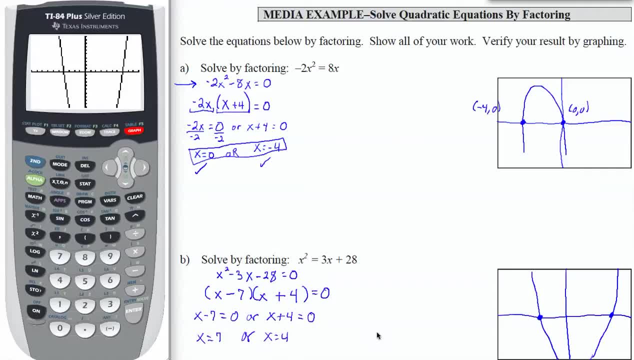 Or x equals 4.. So what I'm betting is that this ordered pair over here is 7, 0.. And what did I do wrong? This should be a negative 4. if I subtract x plus 4 equals 0. So x equals negative 4.. 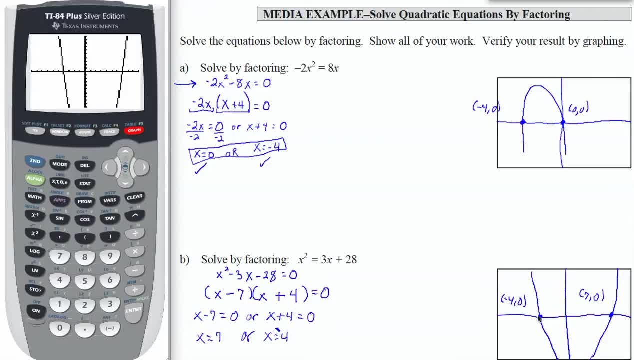 Let's make that correction And I can tell by my graph, So you can see. if you make a mistake here, your graph should help you verify. Now let's go ahead and use our calculator to find these numbers. If I go 2nd, calc 5, that's going to give me one of my intersections. 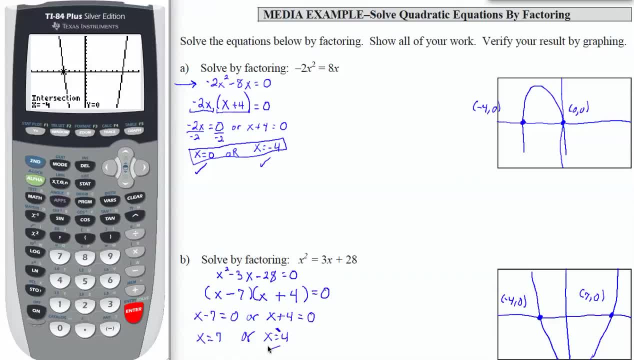 That's going to give me the negative 4, 0.. So this one checks. Let's do 2nd calc, number 5 again, And I'm going to need to move my cursor over until I can get a little bit closer to the. 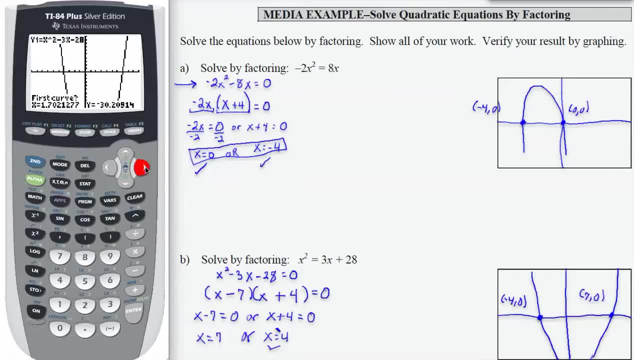 second intersection that I'm looking for. Notice my y values are still going down. Now they're starting to come together. They're starting to come back up. They're less negative. I'm getting into negative 12,, negative 10.. There's my cursor. 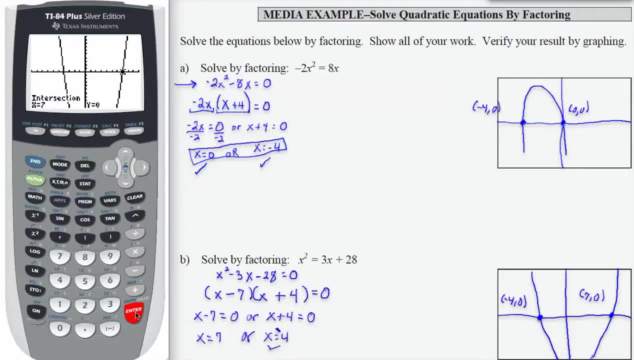 Now I'm going to hit enter 3 times And that should give me 7, 0.. So it confirms the second solution. So I have 2 solutions, just as I did in part a, to this equation, And they are: x equals 7 or x equals negative 4..